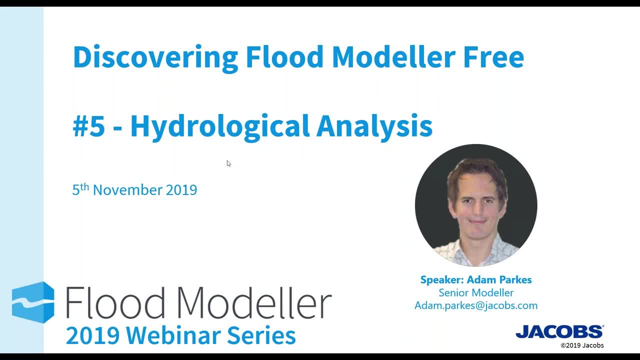 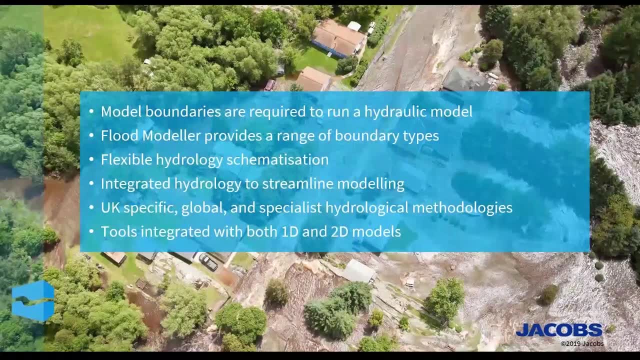 I've been asked to talk to you today about some of the tools available in Flood Modeler for hydrological analysis. So just an overview. you've built your hydraulic model. you've spent a lot of time putting in your cross sections, your bridges, your routing units. 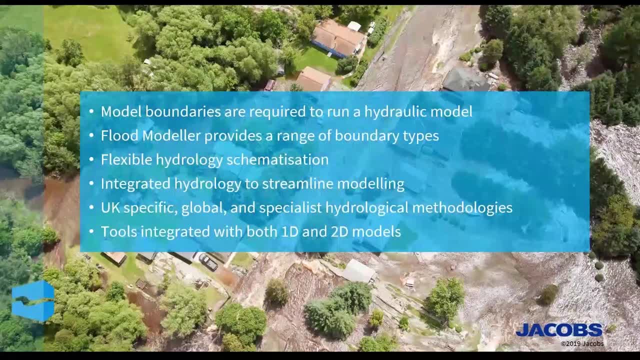 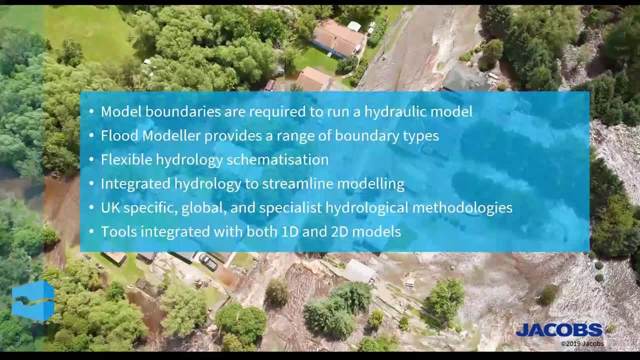 but to really make use of that model you need some boundary conditions. you need some flow to go into your model to drive that modelling process, And that's where Flood Modeler is really great. We've got a wide range of boundary types and systems available, built straight. 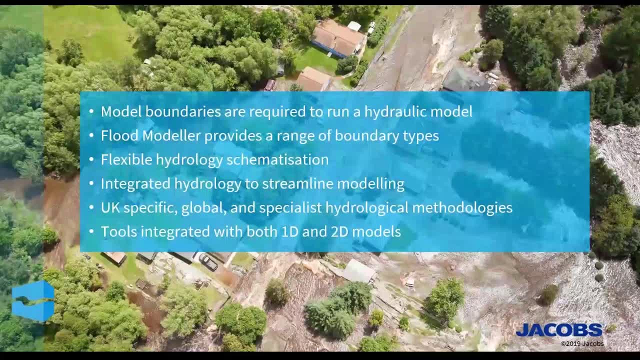 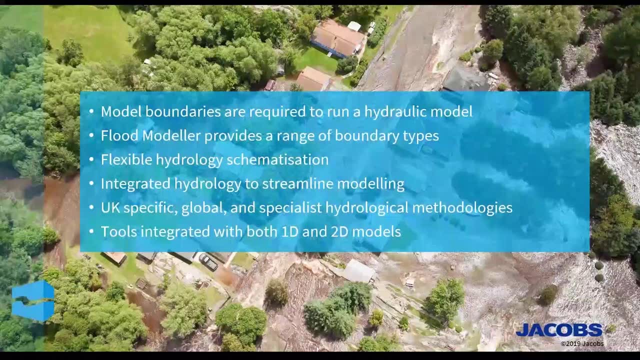 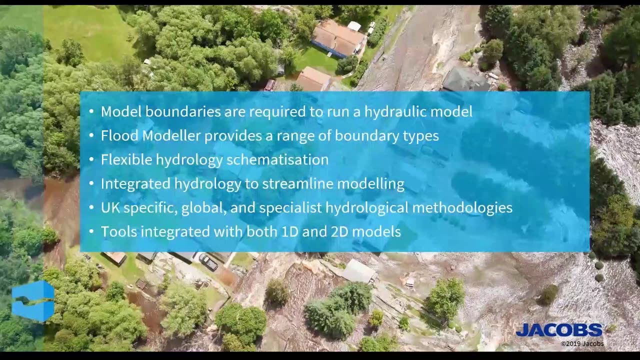 into the software which allow you to easily link up your boundaries, your hydrology, to your hydraulic model and run the model all within one place. So the software is flexible. There's a wide range of ways of schematising the hydrology for different study types and different catchment types. All the hydrology tools are integrated. 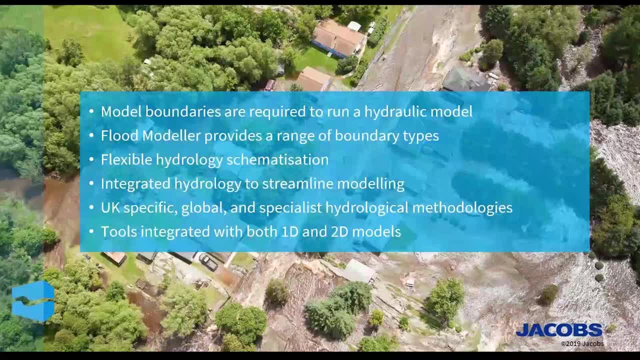 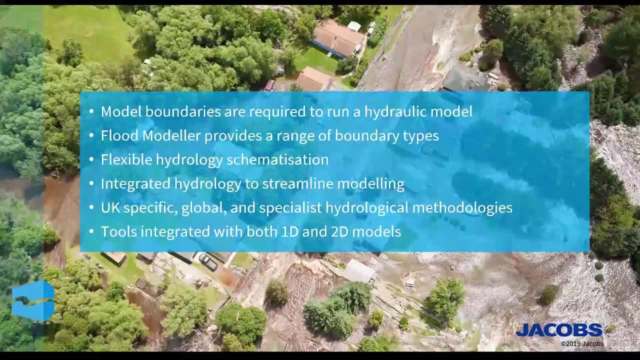 within the software, which brings streamlined approach So you can undertake your hydrology, build your model, run your model and then process your results, all within Flood Modeler. We have methodologies that cover UK specific applications, global applications, as well as a wide range of specialist hydrological methodologies. 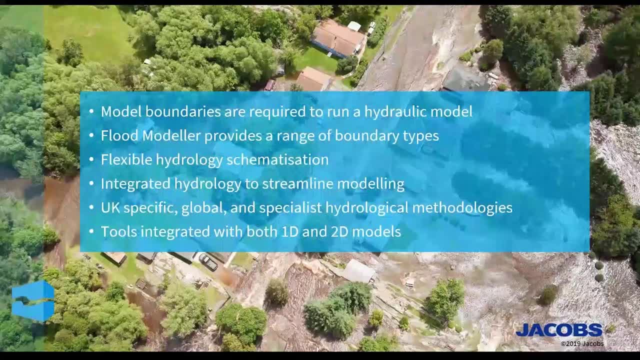 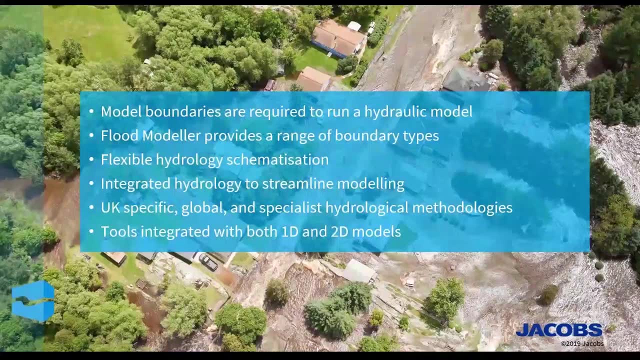 And also one of the great things is everything you do in 1D, so all the boundaries used for a 1D model are applicable to the 2D solvers, So you can easily mix and match between 1D and 2D solvers. So in this presentation I'll be giving you a quick overview of the boundaries. 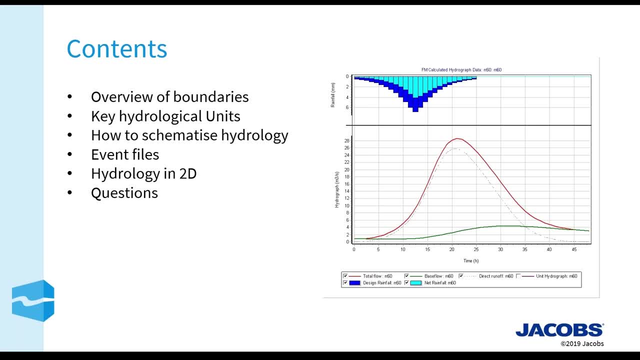 within Flood Modeler what's available. We'll look in a bit more detail at some of the key hydrological units, the ones that are most used. I'll also show you how to schematise your hydrology, so how Flood Modeler allows you to adapt your model to match your catchment. 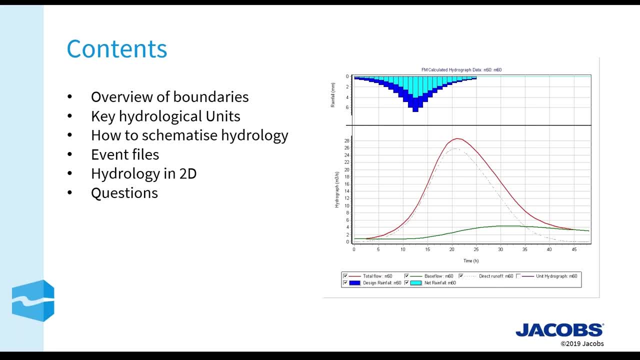 schematisation where the tributaries come in, how flows are distributed. We'll look at event files. These are a key aspect of Flood Modeler, giving you the ability to be efficient in your modelling and file systems. We'll also look at how you apply boundaries. 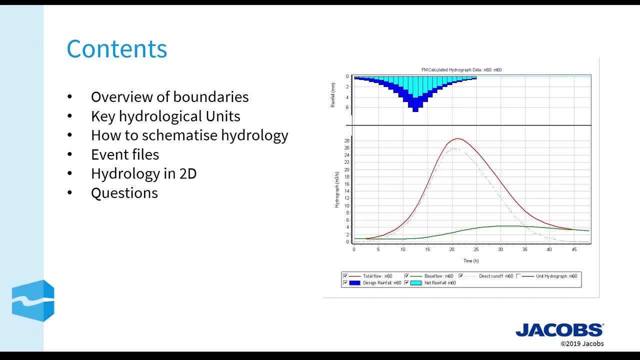 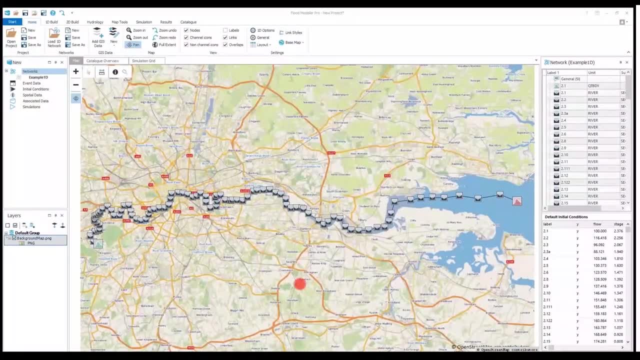 within a 2D model, within a 2D solver using Flood Modeler- And at the end we'll have time for some questions- Flood Modeler interface. So I've loaded up a demo model. So this is the Thames model. 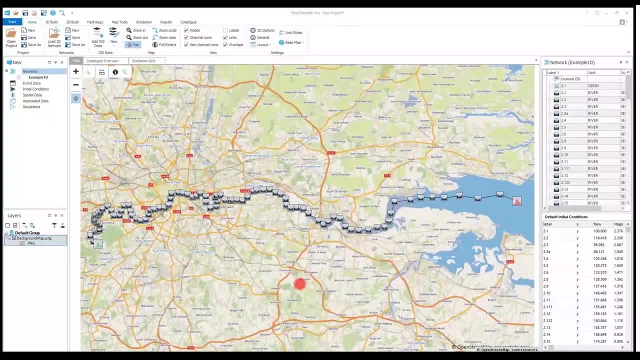 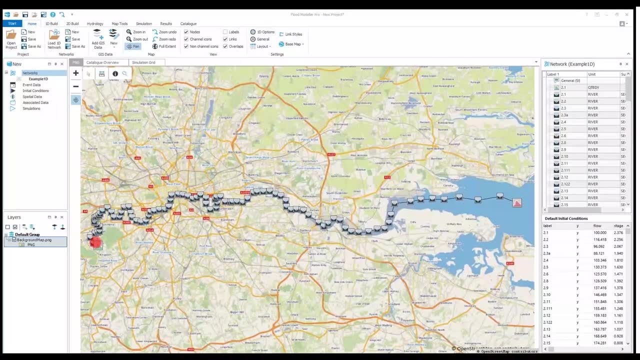 which ships with Flood Modeler. When you install the software, we give you a number of demo models to play with, and this is one of them, So you can go and do these exercises afterwards if you choose. So the hydraulic model consists of a number of linked cross sections, So all 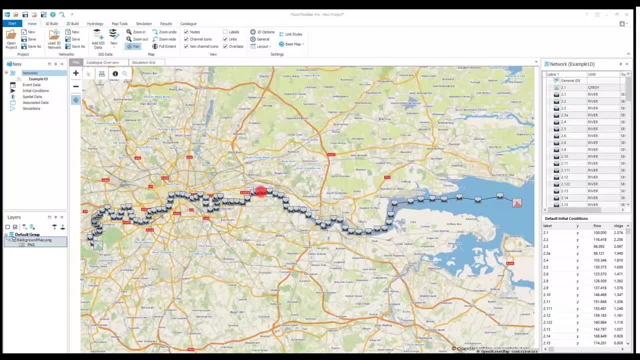 these little blocks running down the channel are the cross sections representing the conveyance of the river system. Under the top we have an upstream boundary, in this case a flow boundary, And the bottom end, on the right-hand side of the screen, where my red dot is, you can 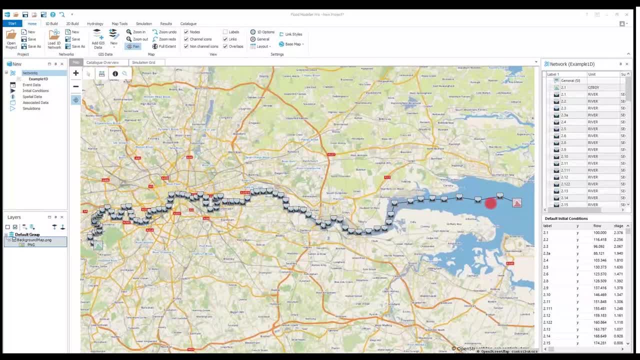 see, there's a downstream boundary, in this case a tidal boundary, because the model discharges into the sea. So what we want to see is: how do we set these up, How do I choose these and what options do I have within Flood Modeler? So, first off, where are all the boundaries? 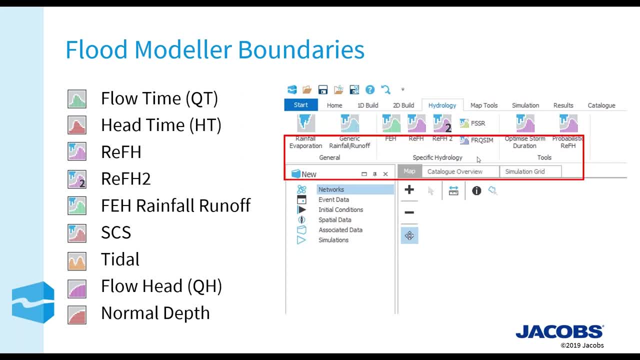 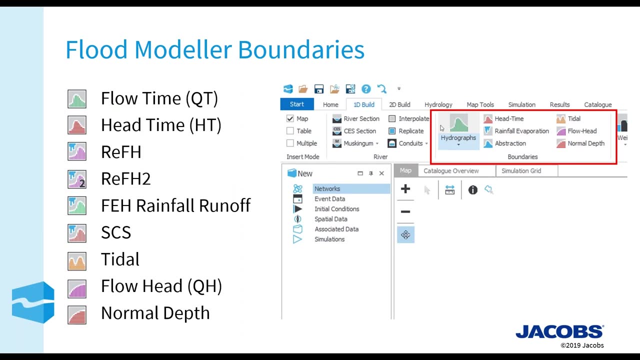 So in Flood Modeler in the interface under the hydrology tab, there's a series of these boundary types we can apply. These are largely the more complex, more involved boundaries like the rainfall rough. In addition, under 1D model build under the boundaries section there's another series. 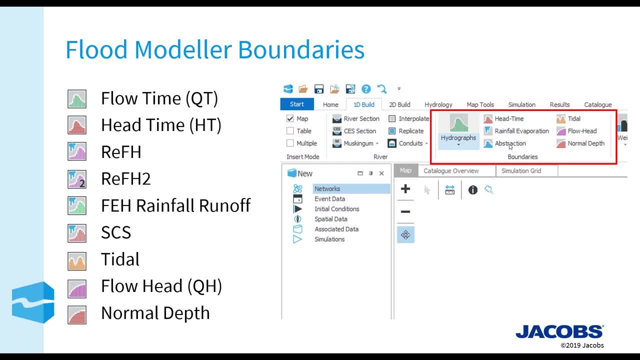 of boundaries available to us. Down the left-hand side I've identified some of the key boundaries which we're looking at, So we've got the flow time and the head time boundaries. These are QT and HT. So the flow time, the QT boundary, is a user-defined flow series over time, So you specify what the 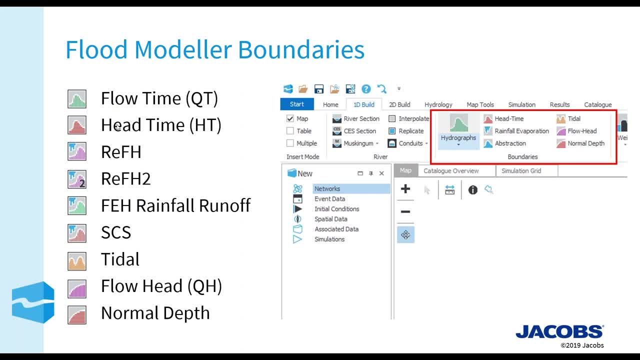 flow entering your model is at specific times, So the flow time is according to the H4 and the flood time boundary values. So what we are going to see is that, of course, you're rather interested in what you're looking at. in the flow, too, There's lots of features we can use to help you identify all of these. 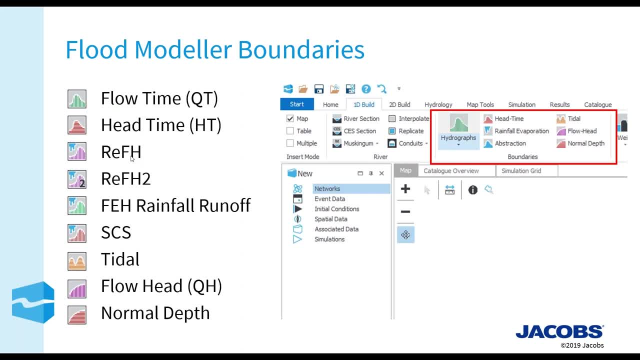 and the utility features you can find in the flow query for your model. In terms of the flood time, we're going to look at exactly where your model isytes And these are the rfh ones, the feh one and the, the generic rainfall runoff for scs method one and. 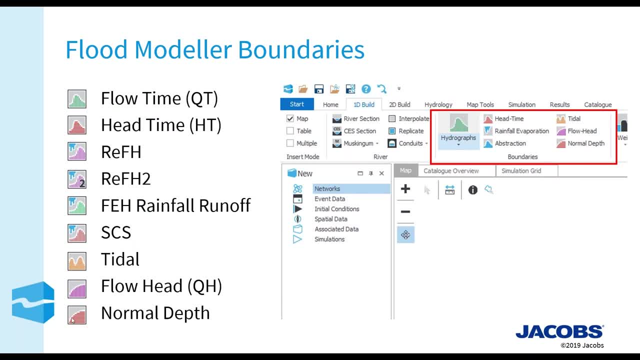 we'll talk about those a bit later on. we also have a good range of downstream boundaries. so these tidal boundaries, qh boundaries and normal depth boundaries i'll come on to shortly- most models at the very least require an upstream boundary and a downstream boundary. so if you've 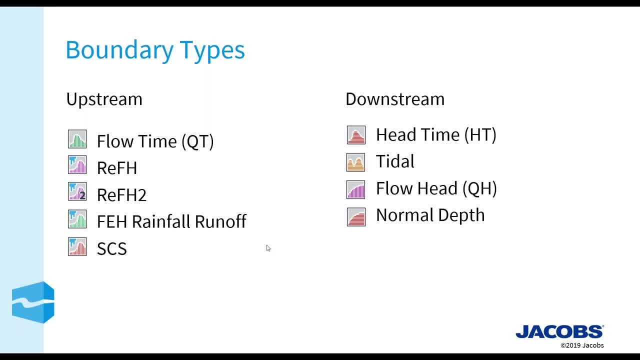 got a single reach, a single series of cross sections or routing units or culverts. you need a flow boundary at the top, so that's the flow coming into your model, and a downstream boundary at the bottom, which is the controlling downstream water level, and generally an upstream boundary. 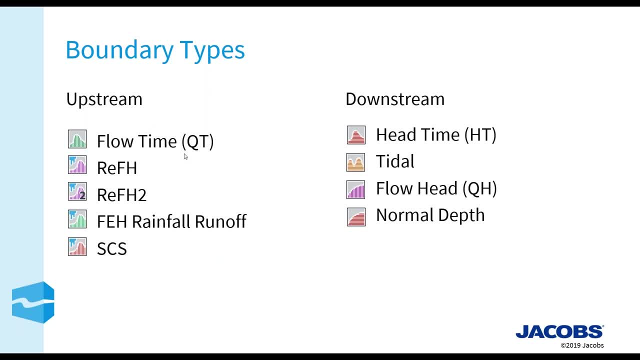 would be either a flow time boundary- this may be if you've got some observed data. so you've got some observed flow data you want to put into your hydraulic model- or some sort of rainfall runoff boundary, so the the rfh, the feh or the scs boundaries where you want to simulate a given. 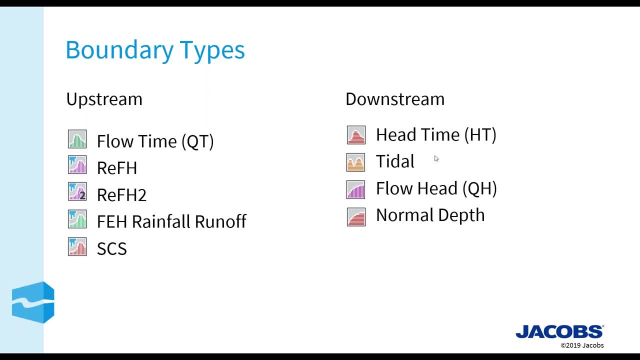 return period event, the one in 100 year- flood event. downstream boundaries really depend on how the model finishes. so what's at the bottom of your model? so if it finishes, say, in a, in the c, you want to use some sort of tidal boundary. so if you either define a tidal profile using a, 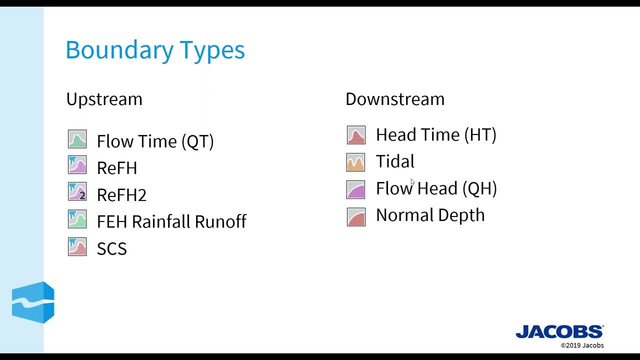 ht boundary or a tidal boundary. we define the harmonics. you can use a flow head boundary, a qh boundary. these are really useful, so what they do is convert the calculated flow in your hydraulic model at the last cross section into a level, and that may be based on the qh relationship you have. 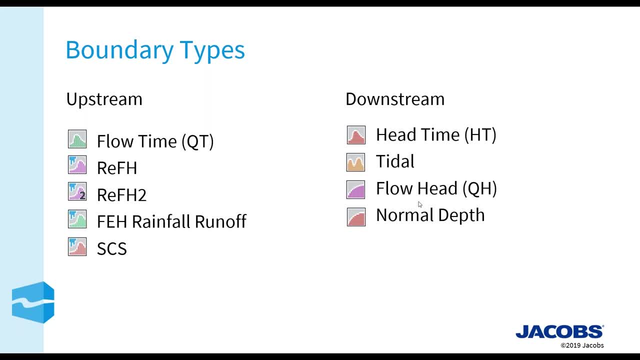 from a weir, say, a gating station or it may be some other flow head boundary you've you've derived. often we use these normal depth boundaries as well. these are effectively continue the hydraulic gradient for your model downstream. so if you're modeling a big river system, so the thames for 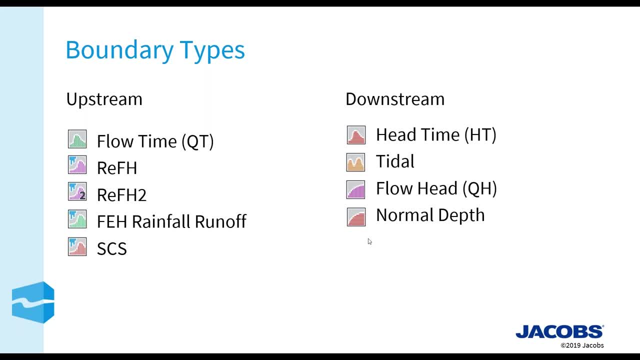 instance, but you're only interested in a small section of it. rather than having to model the whole thing down to the sea, you simply model the section you need and you can apply a normal depth boundary at the bottom of your model which continues the hydraulic grade down beyond your. 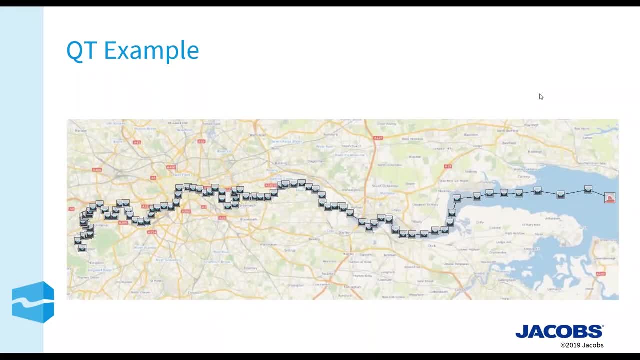 model, reach. so let's look at how you apply these. so i've gone back to the thames model as my example. in this case i've removed the uh, the flow boundary- at the top. so at the top of my model i've got cross sections heading downstream towards the sea and where i've got my my head time boundary. 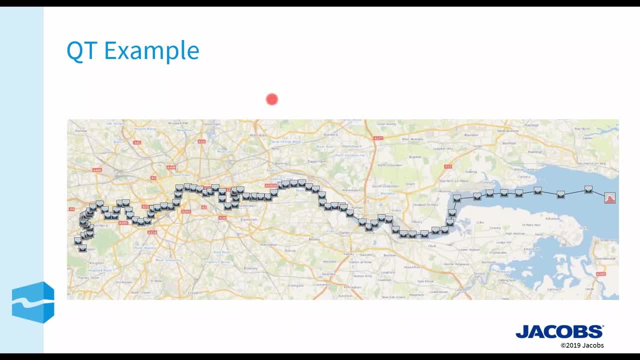 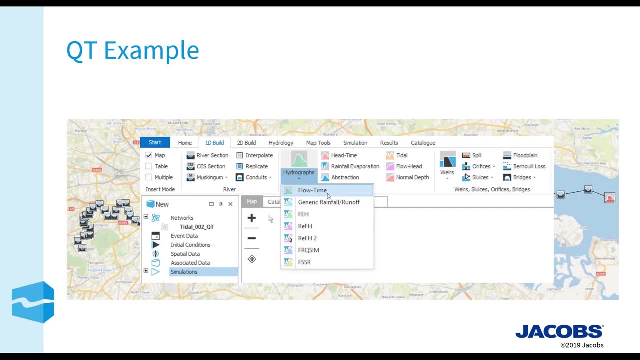 but i don't have a qt boundary at the top of my model, so i need to introduce something. to do this, i simply go to my 1d model build tools under hydrographs. i'm going to select a flow time boundary and i choose where i want to put that in my hydraulic model. so spatially i i select. 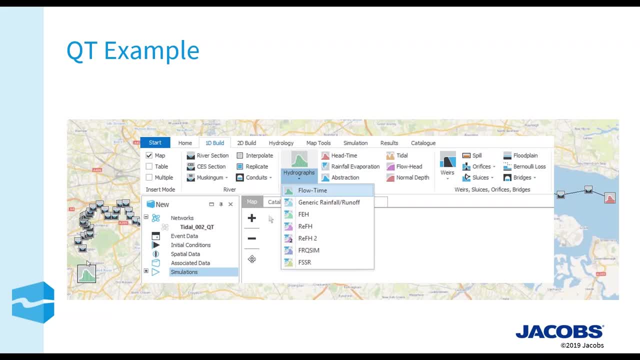 the location i want to place it and just click and that will add my boundary into my model and it's the same with all the other boundaries, whether it be an rfh or downstream boundary, qt boundary and abstraction. just simply choose the right boundary and choose to click where. 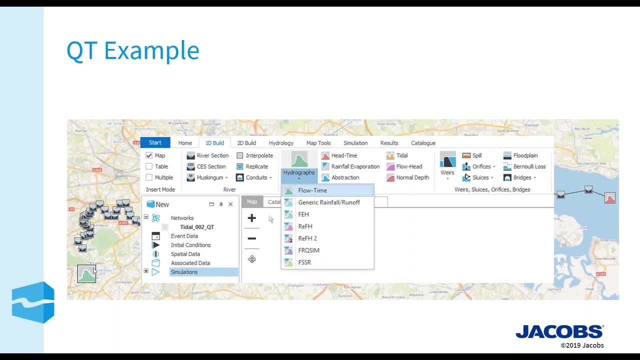 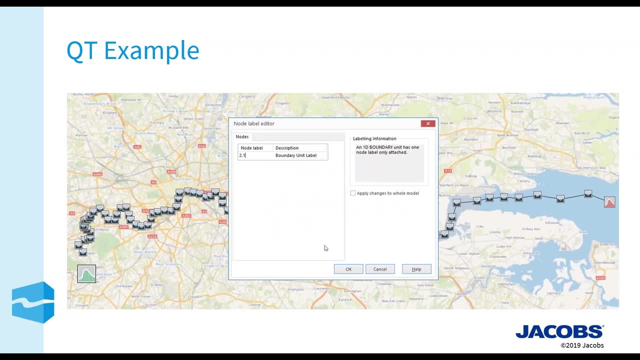 it goes in your network. the way flood modeler knows that that boundary is connected to your cross sections is by naming convention. so when i click i get a pop-up box asking me: what do i want to call that boundary and the easiest way to connect it to a cross section? 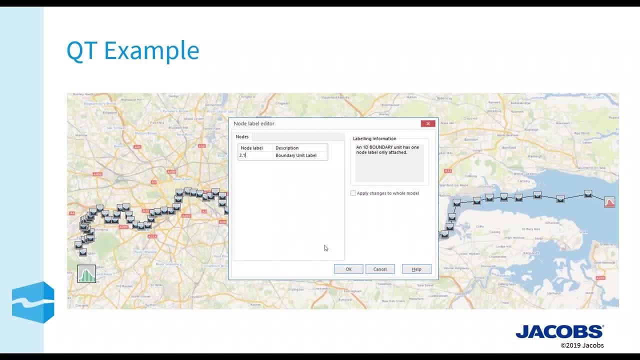 is to give it the same name as the first cross section. so my first cross section is called 2.1. i'm going to call my boundary 2.1 and when i click ok, i get a message pop up saying that that that label has already been used. and do i want to connect the two together? yes, i do so. i click yes. 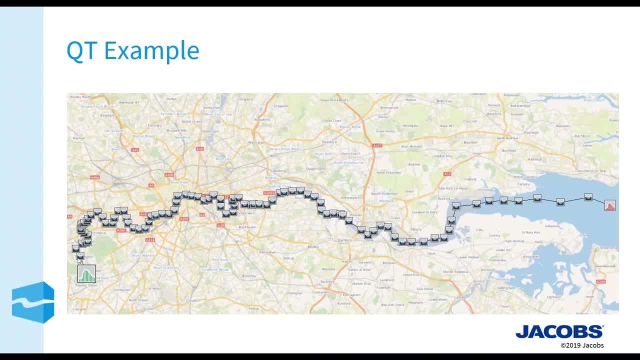 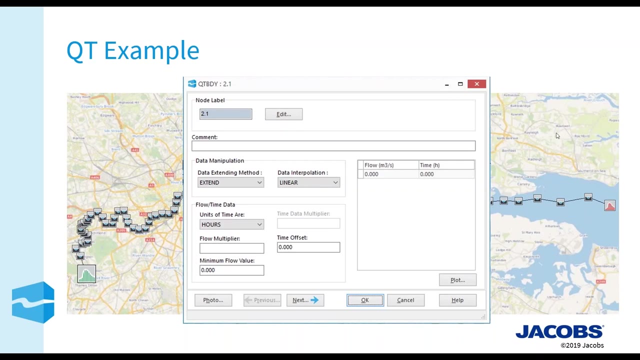 and a little line appears connecting my qt boundary to my first cross section. so now they're linked together on a 3d interface within my qt boundary. so i know that model's set up. i now need to put some data into that qt boundary. so if i double click on that boundary i get the qt interface up here. 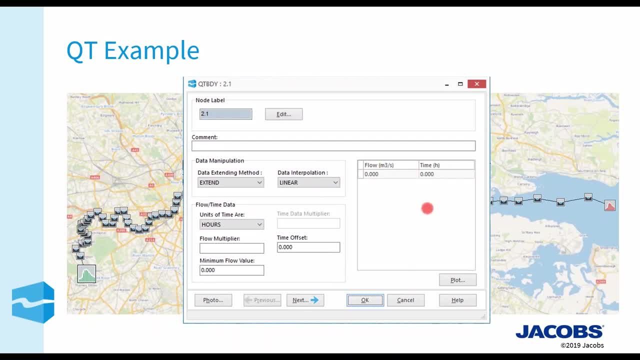 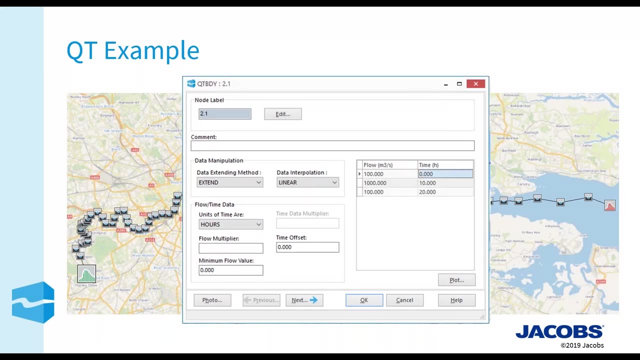 and this allows me to specify some information. on the right hand side i've got my my flow and time information. this is where i specify a flow at a given time. so if i put some example data in here, I've got 100 cumex flow at time step zero, rising to a thousand cumex at 10 hours and then falling. 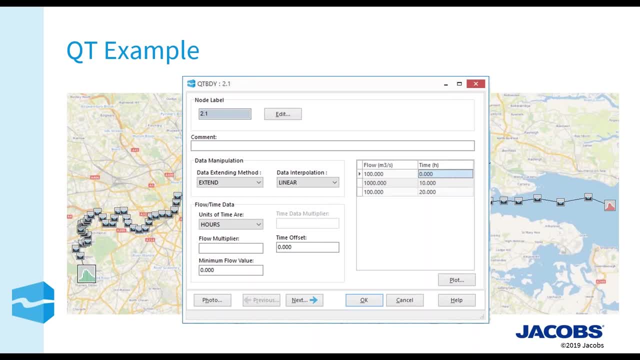 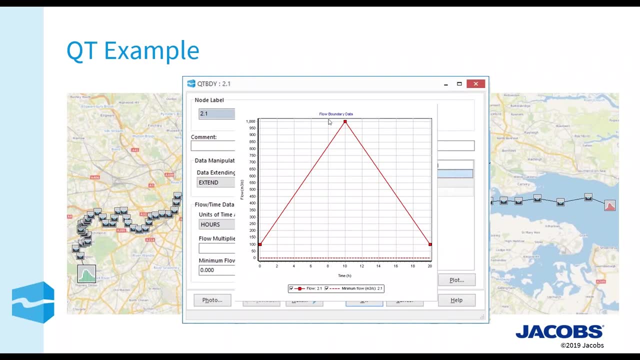 back to a 100 cumex at 20 hours. it's a trapezoidal hydrograph. if I click the plot button, the bottom right hand corner, I can see what that looks like, and so I can see the rise and the fall of the hydrograph over time. I've got a number of other options available to me in the software as well. 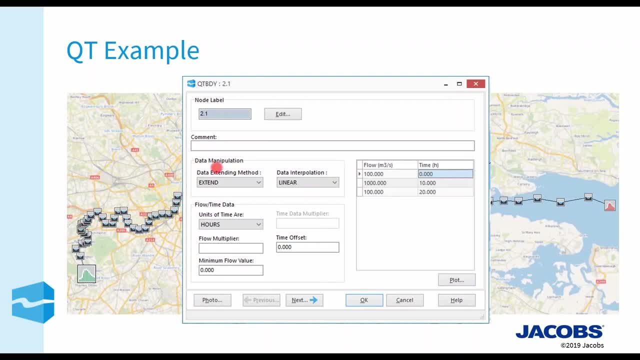 so at the top I've got these data extending options. so my hydrograph inputted only goes out to 20 hours. but if I want to run my simulation for 30, 40, 50 hours, the model needs some sort of boundary data. so by choosing extend and linear, it will take that final value, that 100 cumex and 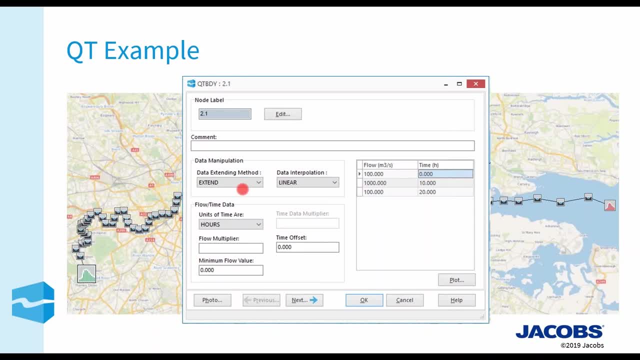 extend it out beyond the data inputted to the extent of my simulation. below that, I've got a number of other options available to me in the software as well, so I can see the. I can specify the unit of time I'm using. we default to hours normally and that's usually. 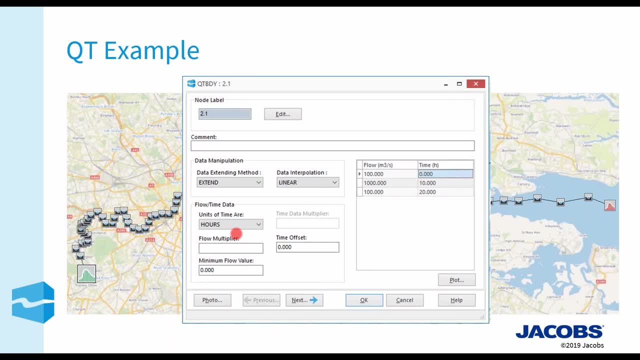 fine. but flood model is adaptable. you can have everything from seconds through to years or lunar months if you wish. the flow multiplier box is really useful. so if I want to test my model for climate change, for instance, I can put a multiplier in here. so if I want to look at 20%, 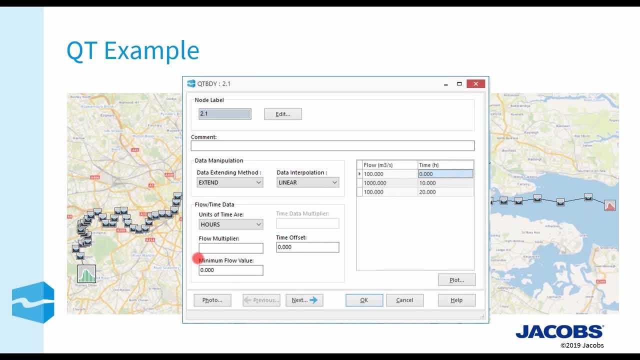 increase in flow. I can simply add in 1.2 in there and all my ordnance will be multiplied by that factor. the time offset box allows me to delay the start of my hydrograph. so if I want to delay my start my hydrograph by an hour or two, I can just put a value in there and it will delay the. 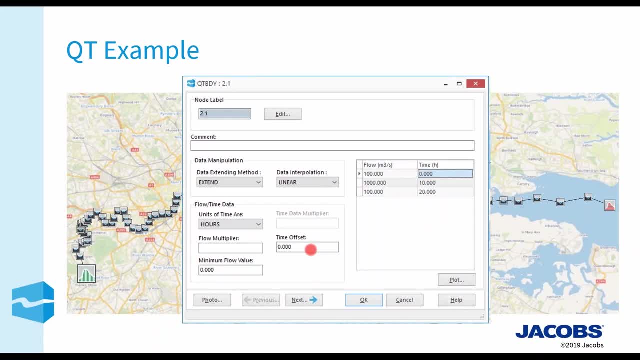 start of that hydrograph by that amount. and this is useful if you're looking at the phasing of different boundaries. I've had multiple fluvial boundaries or tidal boundaries. I could look what happens at the phasing by delaying or accelerating the start of my hydrograph. 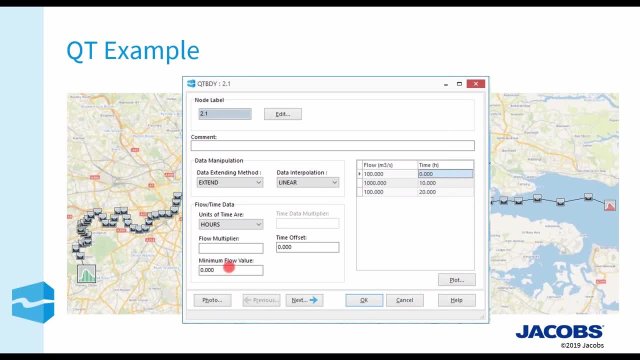 you've also got a minimum flow value box in here. This is useful if your hydraulic model is most stable with a given minimum flow value. So if it's very stable, let's say at one QMEC, and you don't want the inputs drop below that, you can specify a minimum flow in here and that will override. 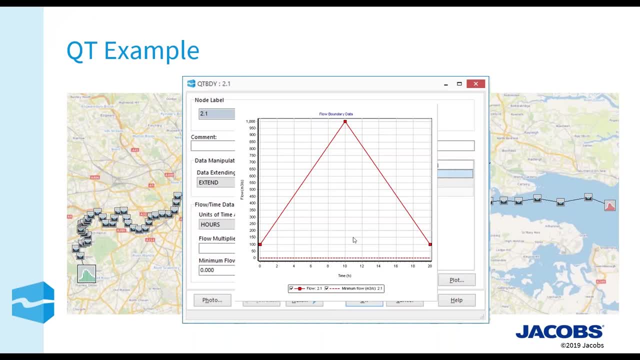 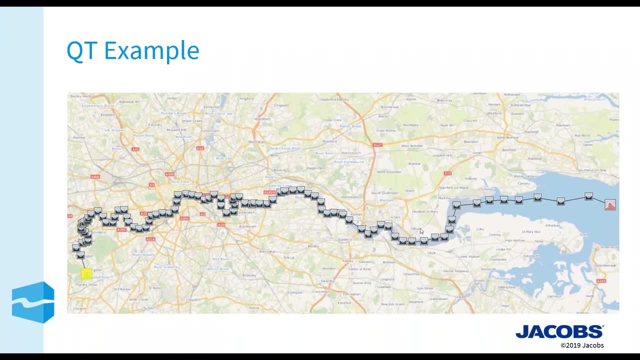 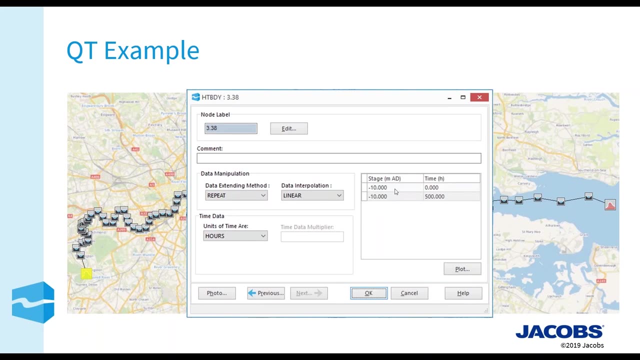 the input data. In this hydraulic model I've also got a downstream boundary, that HT boundary down in the sea. If I double click on that I get a similar interface box. In this case I've specified a constant level, So I've got minus 10 meters for a full 500 hours. So 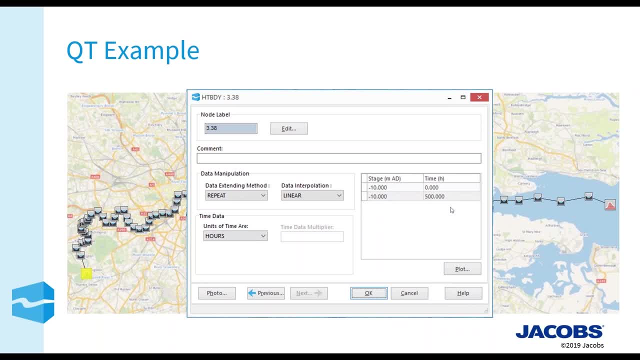 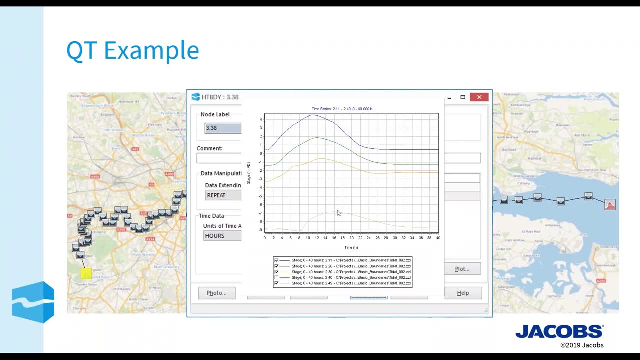 without the entire simulation there'll be no tidal profile at all. The system's got a free discharge. If I run that model unsteady, I can look at some results. So using the new plotting tools in Flood Modeler, I can choose several cross sections and plot them in one go. 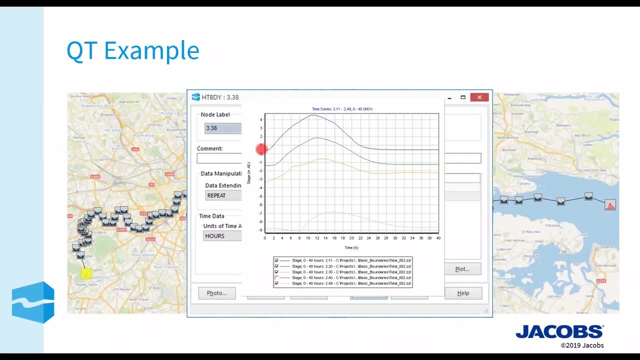 And I can see the stage profiles that resulted. So I've got the blue line, which is the modeled stage profile, at the top of my model, moving down to the line at the bottom, which is the stage profile far closer to the tidal outfall, And I can see things that have been modeled as. 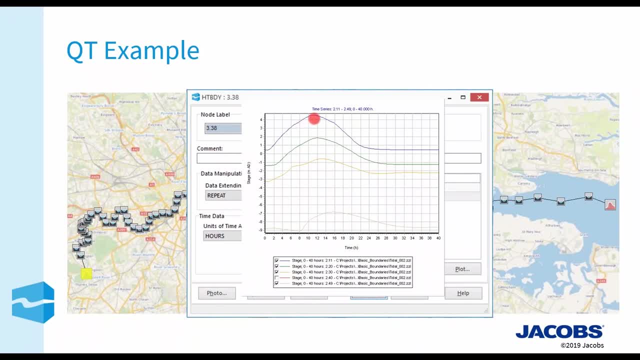 expected. So at the top of my model my hydrograph peak is about 11 hours And as I work through my model, that is delayed due to the travel time of the flow hydrograph And the level drops with a hydraulic gradient of the hydraulic model. So that's all worked. 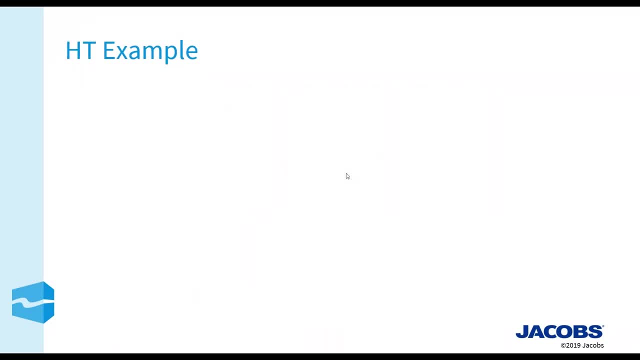 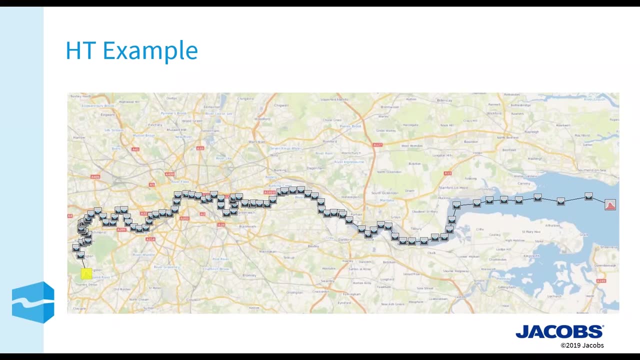 perfectly. That was looking at the upstream boundary in particular. But if I want to have a look at the downstream boundary, same example, But this time I've got a constant flow in my QT boundary at the top, But I'm going to have a tidal boundary in my downstream boundary. So 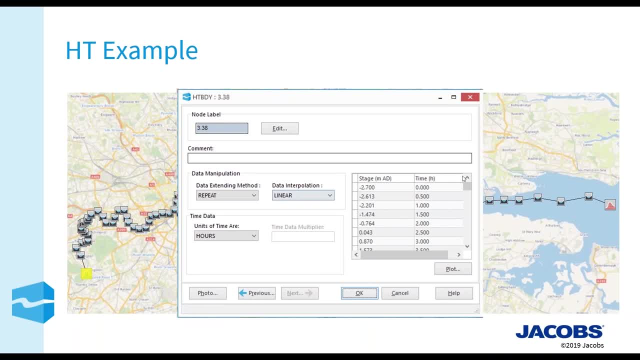 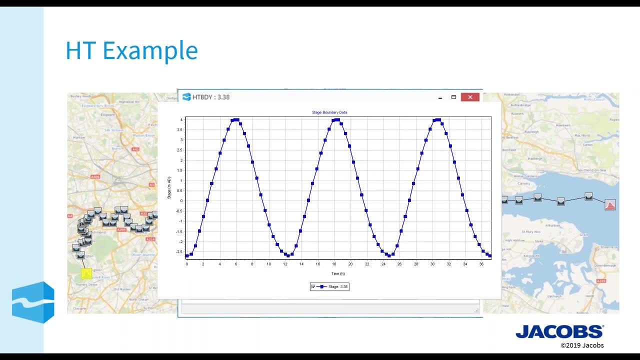 I double click on the HT units And I get the interface box. You can see I put a lot more detail in the the HT information here. So I plot that I've got a tidal hydrograph, So I've got three cycles of peaks and troughs. 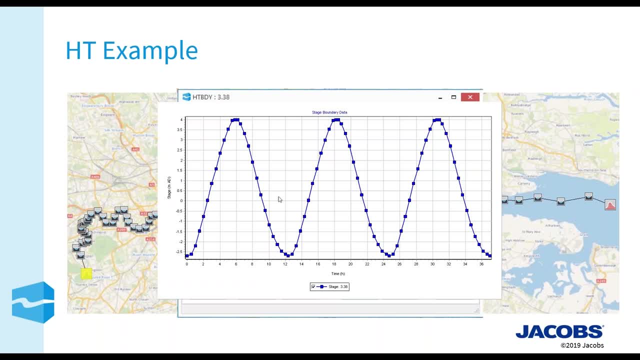 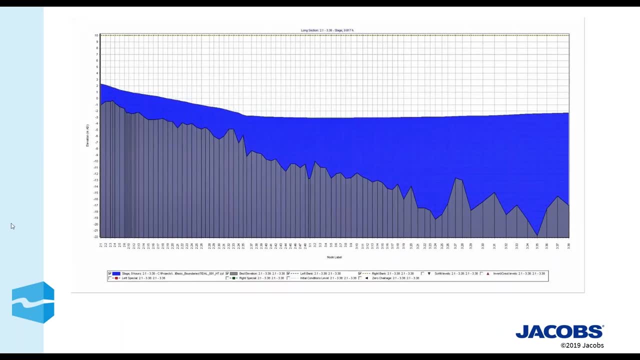 If I run the model now, I'm going to plot a long section. So I choose all the cross sections of my model and plot them. And a nice thing I can do with a flood model is I can animate these So I can see the tidal propagation. 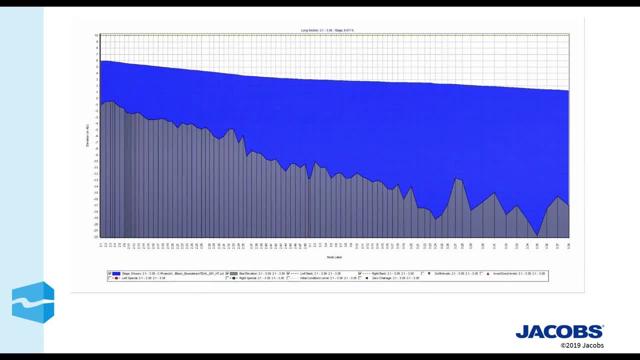 So the tide rises at the bottom of the model and that propagates all the way up through my model And that goes through three cycles of rise and fall. These are easy to generate, So you can use these animations very simply. There's a little record button within Flood Modeler which allows you to export these. 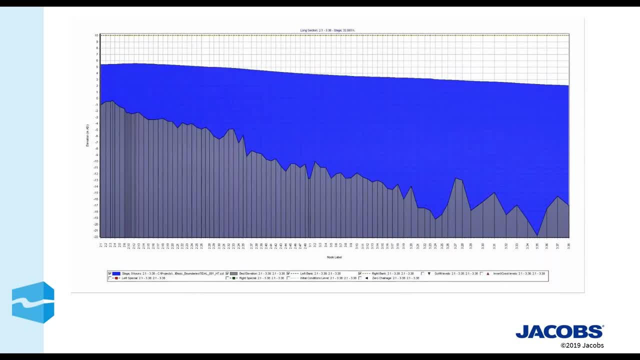 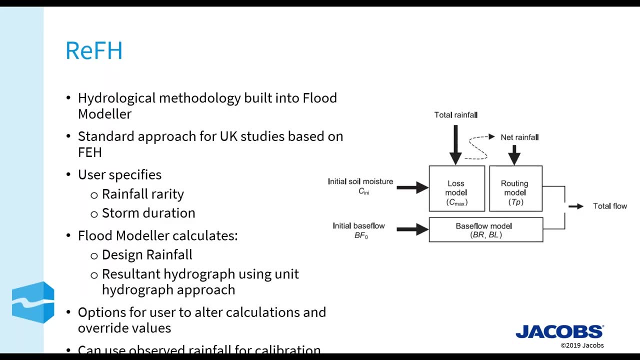 these animations. So that was a quick overview of how you you set up your boundaries, how you attach them, And we looked at QT and HT boundaries. so the other boundary we use a lot are the rainfall runoff boundaries. These are boundaries where the user specifies some rainfall information, so a rarity and a duration, and the software calculates a resultant. 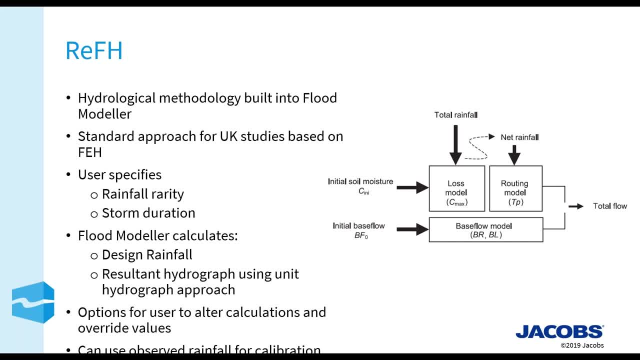 flow which will be discharged into your hydraulic model. And this is based all on the, the catchment form, so the catchment characteristics: how big it is, how steep it is, how permeable it is. The most commonly used of these is the RAFH unit, so UK centric units. 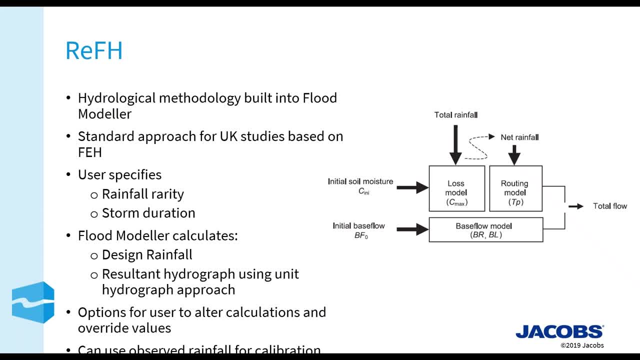 And we talked in a lot more detail about this unit in a previous webinar, which is available on our website. if you want to get more information, Really, all you need to know is the: the user specifies the catchment descriptors and the rainfall data and the software calculates the flow which comes out of that unit. 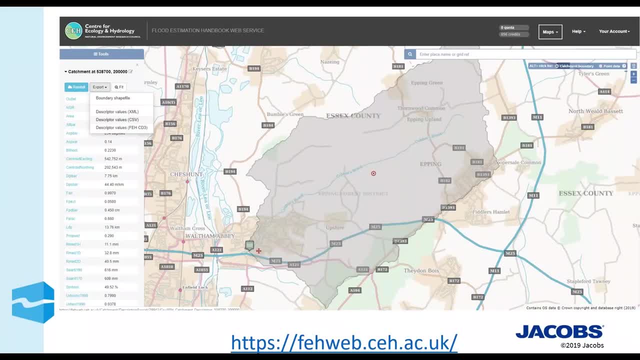 looking at how that works. we get our catchment descriptors generally from the CH centre for ecology and hydrology web service. this is a paid for service, so you you register an account, you choose your site of interest and you click to highlight your, your catchment, and that generates. 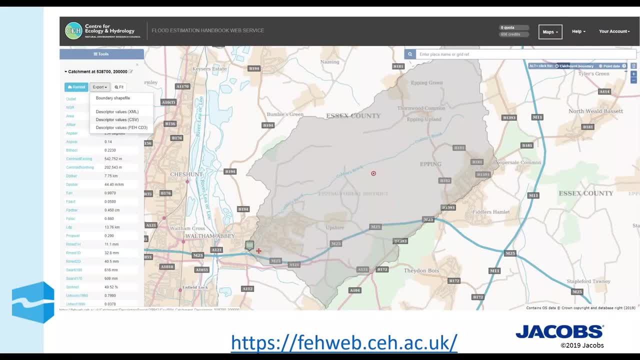 your catchment descriptors for you that tell you how big the catchment is, how steep it is, how permeable it is, how much rainfall it receives, and we can export the catchment descriptors as a csv file using the export tool. that csv file can then be imported directly into flood modeler. 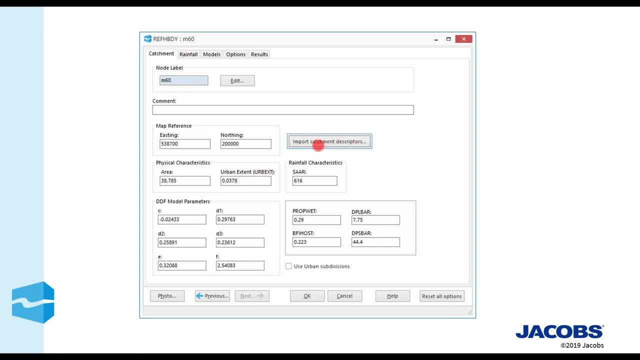 so there's a import catchment descriptors box right in the center of the rfh units and that's brought in all these catchment descriptors. on the next tab we can specify our rainfall. this can work either as designed or as a custom design, and that's what we're going to do today. we're going to go ahead. 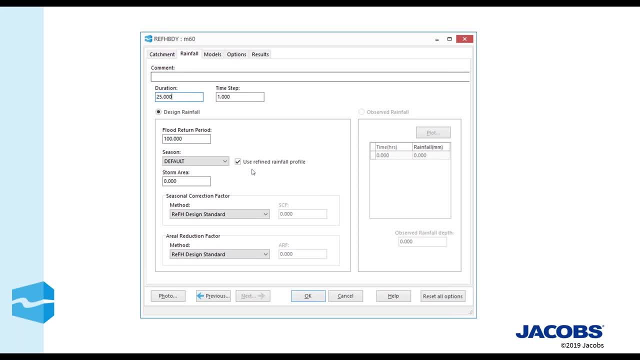 and assign rainfall. so in this case i've specified a storm duration of 25 hours and a flood return period of one in 100 years, one percent aep, or alternatively i could have input that information as observed rainfall. so if i'm trying to replicate an observed rainfall event, i could get observed. 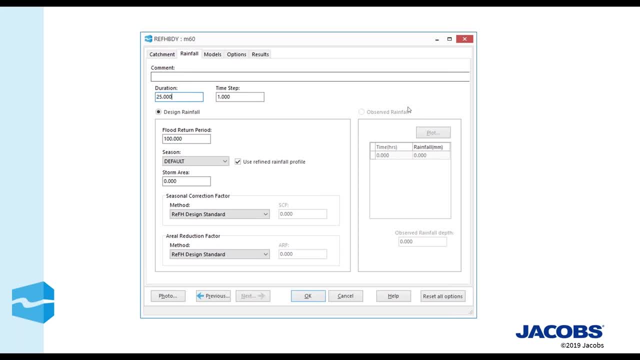 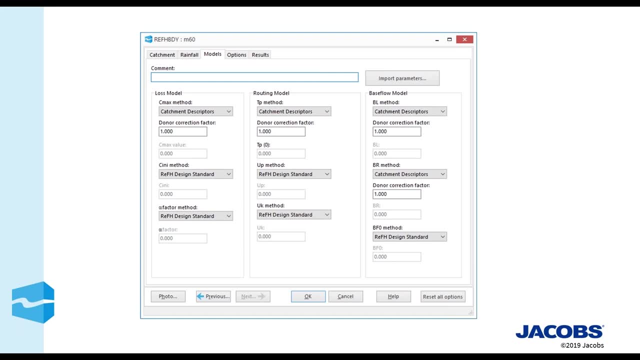 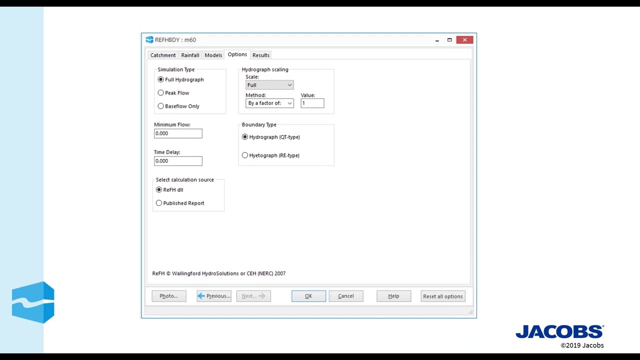 rainfall data from a gating station, simply paste that in there and use that instead. flood model gives you full access to all the different parameters and settings within the rfh unit, so under the model tab and the options tab- and again, we go into a lot more detail about these in the previous hydrology webinar. 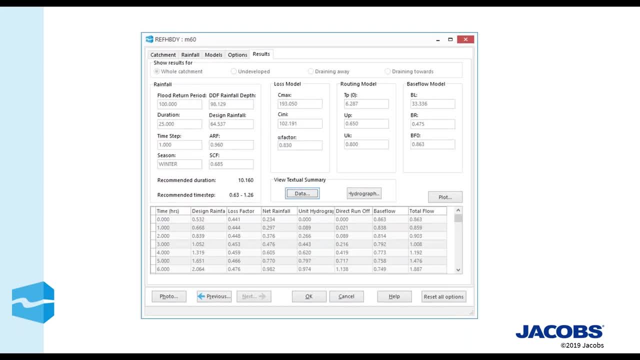 what we're interested in this one is the results. so if I click on the final tab, I can see the software has churned through and it's generated me a hydrograph for my input rainfall. the best way to see this is to click the plot button and I can plot up that. 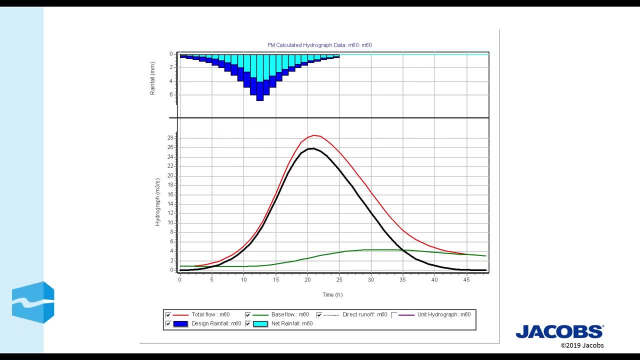 data so I can see I've got my rainfall at the top of the plot. this is my height graph and that shows the generated design rainfall for a one in 100 year 25 hour storm, and then the red plot below is the resultant hydrograph. that's the flow that's going to come out of this unit and be introduced. 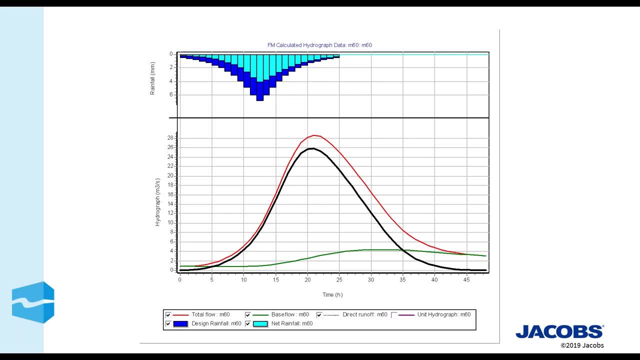 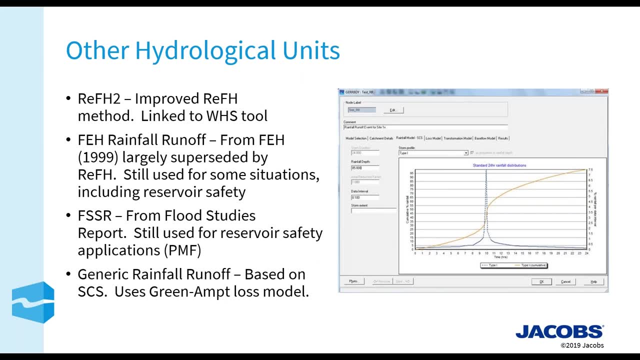 to my hydraulic model. it also shows me the response of both the instantaneous rain runoff and the base flow components in black and green below. in addition to the rfh unit, there are some other rainfall runoff units within flood modeler. there's the rfh2 unit, which is the improved version of rfh, which is links directly into 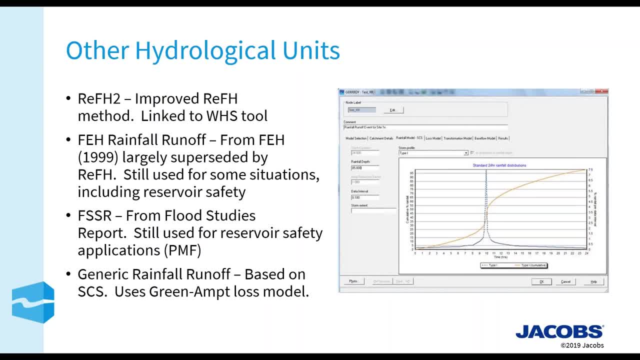 the whs tool. we've also got the slightly older feh and ffsr rainfall runoff units. these have largely been superseded by rfh and rfh2, but they still have good uses for reservoir safety situations. if you're looking at the probable maximum flood or the one in ten thousand year. 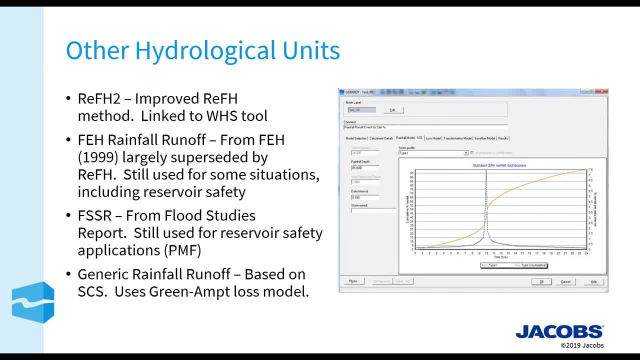 flow to go into your reservoir for safety purposes. these are the units you tend to use. we've also got the rfh2 unit, which is the improved version of rfh, which is linked directly into the whs tool. there's the rfh2 unit, which is the improved version of rfh, which is linked directly into the whs tool. 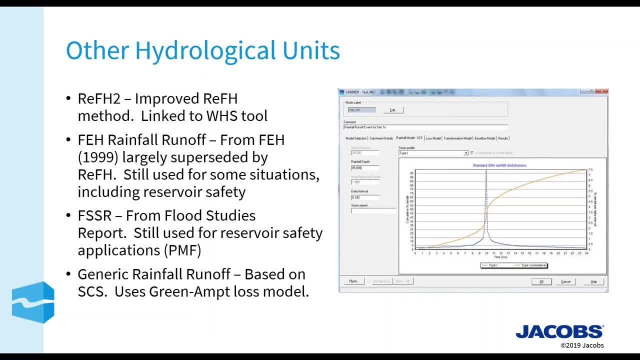 we also have the generic rainfall rough units, uh, this often uh called the uh, the scs method. so this is a really adaptable tool which uses international uh methods where the user can specify the different components which make up, which make up the rainfall runoff tool. pardon me, and so i can either use the scs, the sole conservation service. 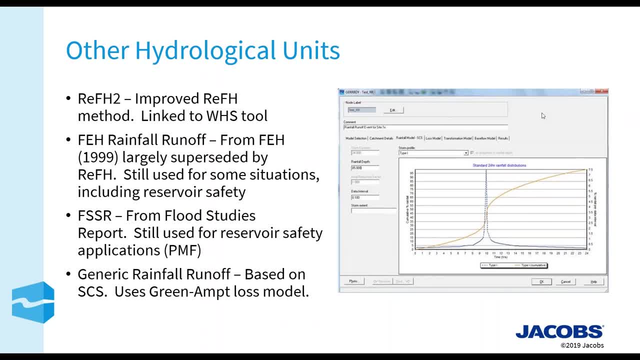 methods or it can use the green out methods and you can mix and match for the uh, the uh, the inputs, the loss model and the routing model. this has been hugely improved in the last few releases of flood modeler and there are some further great improvements coming in the next release. we're also looking to add more hydrological units to the software. 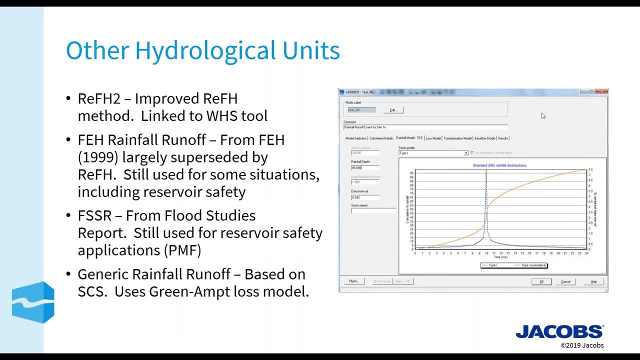 so, for instance, we're looking at implementing the new irish uh hydrological units and methodologies in incoming releases and if there are methods which you think flood modelers should be having, please let us know about them. we've got feedback forms and methods of contacts on our website. 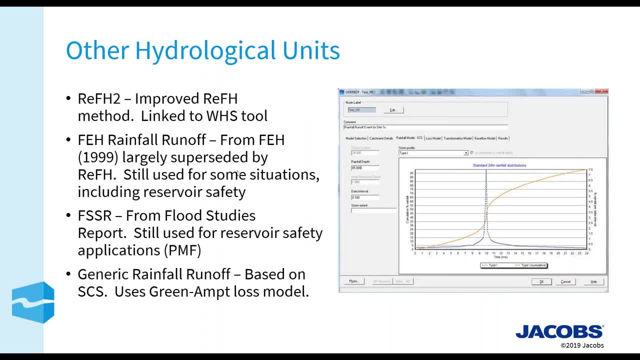 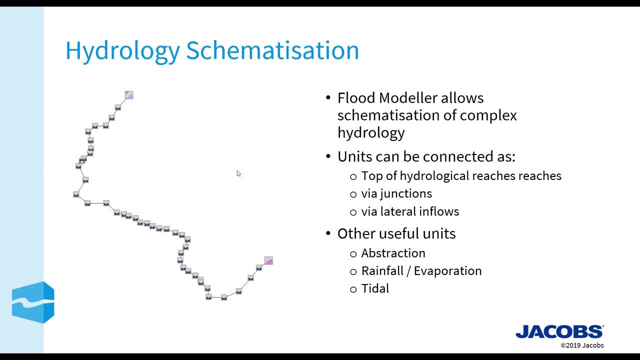 and we've also got a link to the scs model, which you can find in the description. so you've got your, your hydrological units, you've got your rfh or your scs methods and you want to attach them to your model, in addition to the fairly simplistic approach i showed at the start. 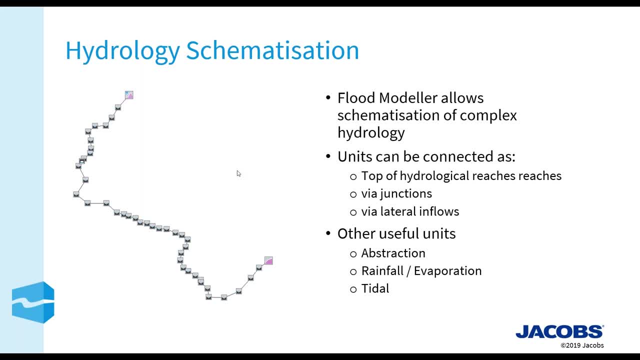 the software is flexible enough to allow us to have different ways of connecting our units up. so in this example i've got um, a hydraulic model made up of cross sections moving from the top of the screen down to the bottom. at the top i've got an rfh unit and the 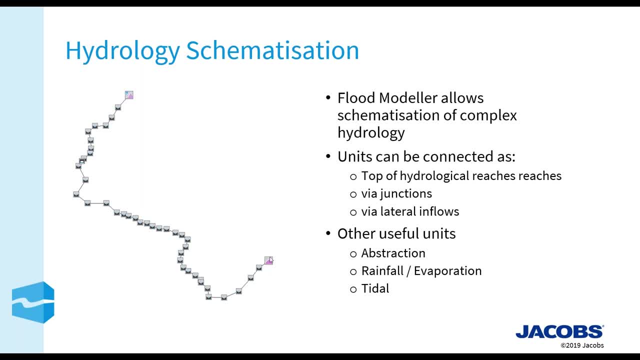 bottom. in this case i've got a qqh unit. if i want to attach an additional inflow, say where i've got a tributary joining my model, i can do so. the easiest way of doing that as a point inflow is to add a junction and i can directly attach 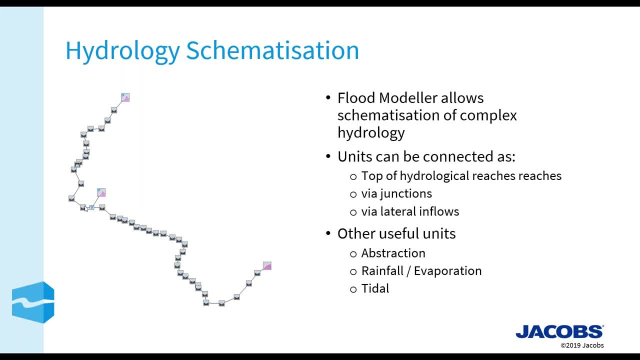 another rfh unit onto that. so i've got my info at the top and my inflow for a tributary midway through. another common way of attaching units is to use the lateral inflow tool. so this is where you want to spread your inflow across several cross sections and this is this used extensively and is very useful. 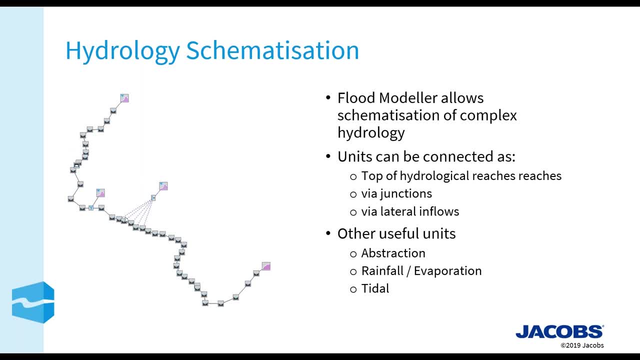 way of doing it. so, rather than attaching your inflow directly to a a model node, you attach it to a lateral inflow unit which then spreads the flow across several cross sections, and the user can define how that's done, but by default it's done based on the 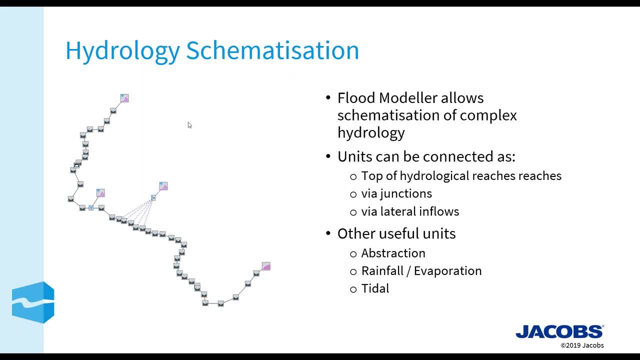 reach length between each cross section. you can apply these methods using all the units we've we've looked at so far as well some of the more specific ones, like the abstraction unit and the rainfall evaporation and tidal units as well. by using these tools, you can end up with 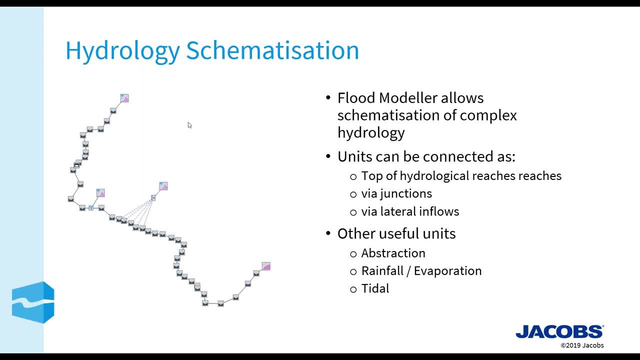 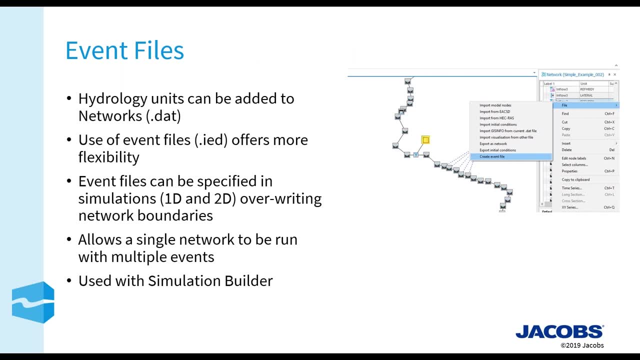 quite complex hydrological skewmatization which best matches your study area and the projects you're undertaking. another great element of flood modeler are the event files. these have been in flood model for many years, but some people are perhaps not fully aware of them. what they let you do is build a. 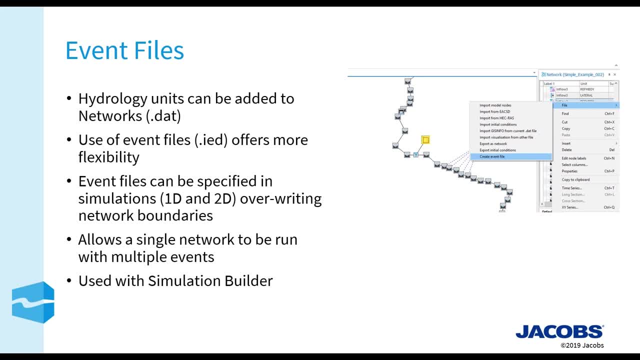 network, a data file, but then you often want to run that for multiple return periods and multiple scenarios, want to have to have a network for every single return period. that introduces the risk of error creeping in and replication problems. so instead you have one network and you have multiple event. 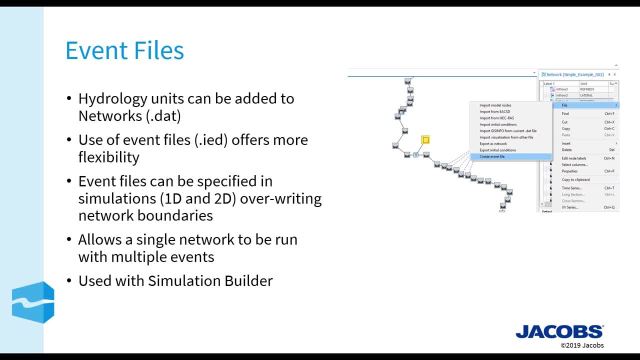 files and the event file. the iid file contains the hydrological units. they're really easy to use. you simply select the hydrological units in your hydraulic model. you can right click on them and choose, create event file and then they're saved out as a little sub model. this, this event model. 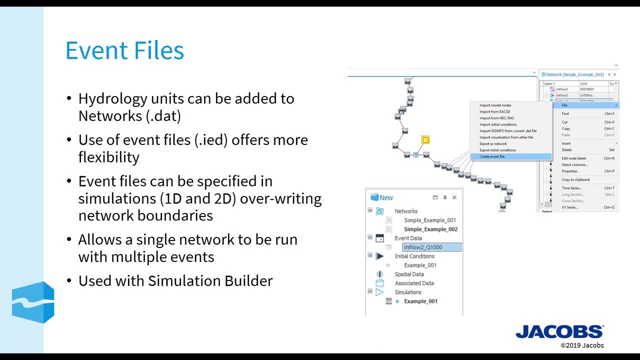 you can then change those event files so you can change the return period, the storm duration, the tidal interaction and so on. and then when you build your simulation, you specify your network and your event file, and any boundary data from the event file overwrites the, the network file. these 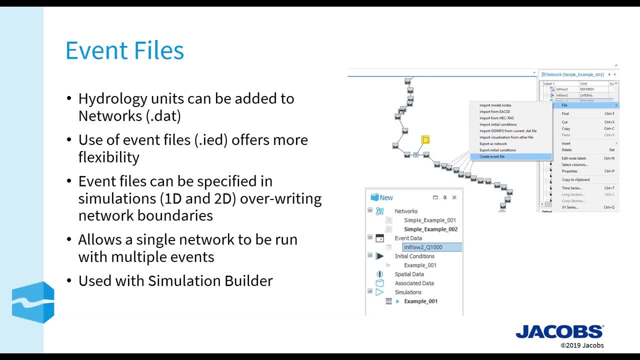 work incredibly well with the new simulation builder. so you build your network, you have a big folder full of different event files, different return periods, and the software will automatically create for you all your simulation data and then you can then create your event file, and then you can then create your event files, which you can then feed directly into the, into the batch. 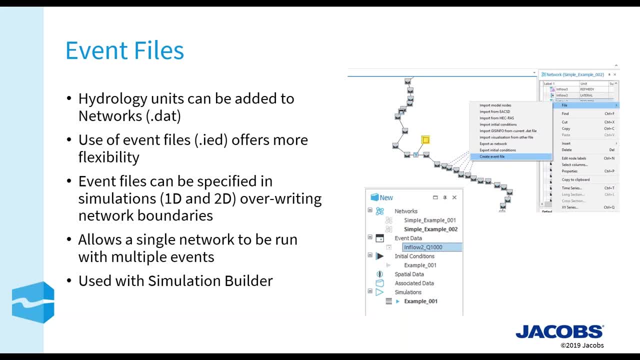 simulator or flood cloud to run your simulations. it makes handling lots of different simulation types a lot easier. another great thing with event files is they're not limited to hydrology units. you can use them with any unit, so bridges are a good example. so if you've built your network and you 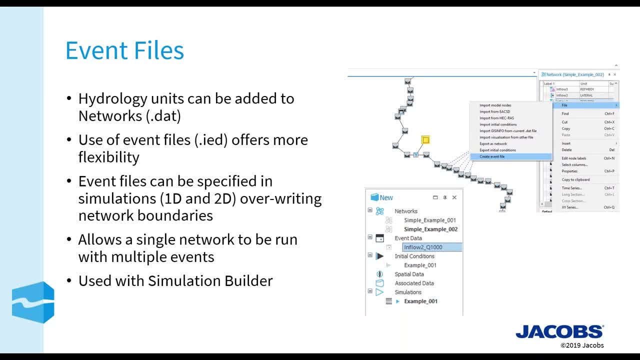 want to test different, different bridges or different blockages. you have one network file and a series of event files, each with a different blockage percentage, which you can swap in and out of your hydrology unit, so you can use them with any unit. so bridges are a good example. so if you built 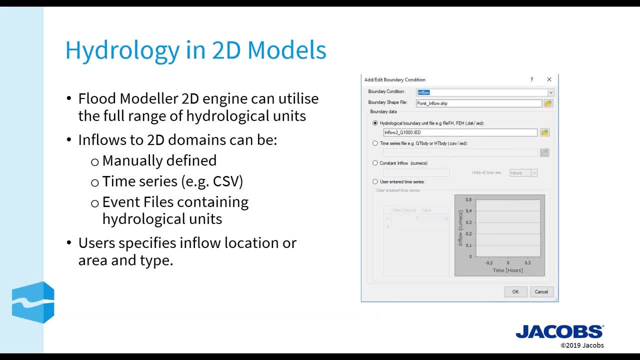 your network. you can use them with any unit. so bridges are a good example. so if you built it model, as I said at the start, flood model is good for swapping between 1d and 2d solvers readily. so when you set up your 2d model, you can. you can apply boundary in a range of different. 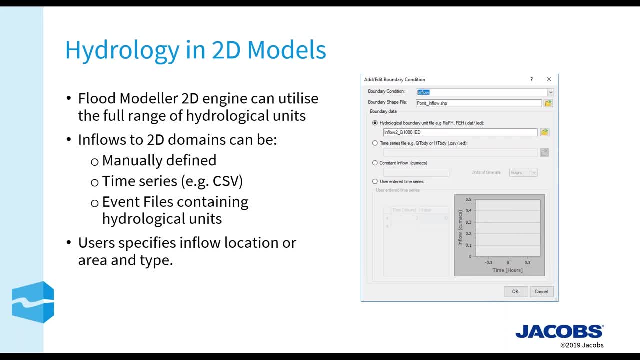 ways you can manually define them, so a fixed inflow or a fixed discharge. you can use time series data so you can import csv files with observed flow, observed level, or you can reference event files. so if you set up your hydrology in in the 1d solver, you can use those event files to 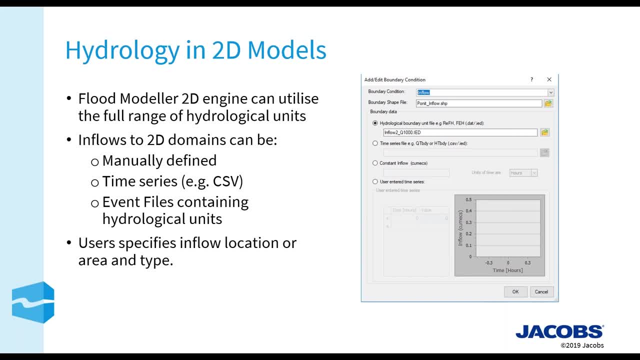 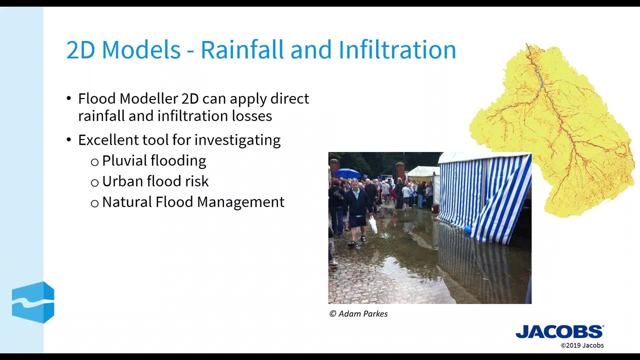 reference event files as inputs into a 2d model. it's incredibly easy to do. you specify the location you want to apply that boundary point, the software at the event file and press go and the software will run through. another advantage of 2d models is the ability to use direct rainfall modeling. so 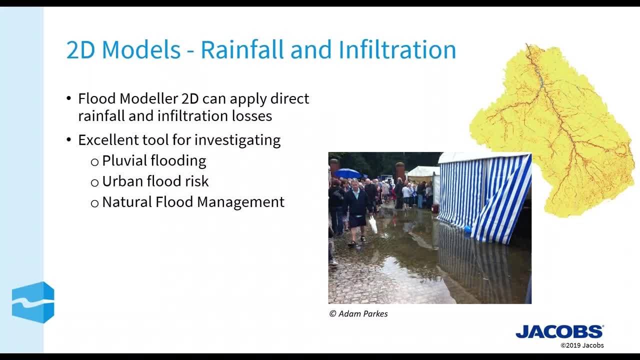 if you're looking at pluvial flooding, if you're looking at urban flooding or looking at natural flood management options. these are very useful so you can build your 2d model of a catchment and that can range from something quite small, so a small scale catchment of a town or a village, all. 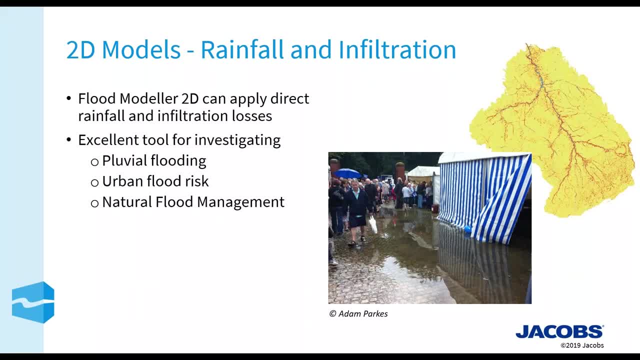 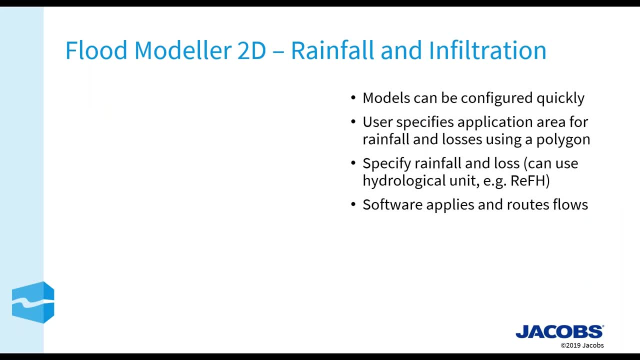 the way up to modeling entire catchments, and you can drop rainfall directly on top of it using our tools. the user simply has to set up the 2d model, specify the area over which their rainfall is applied and then give the software the rainfall data to apply to the hydraulic model. it's worth. 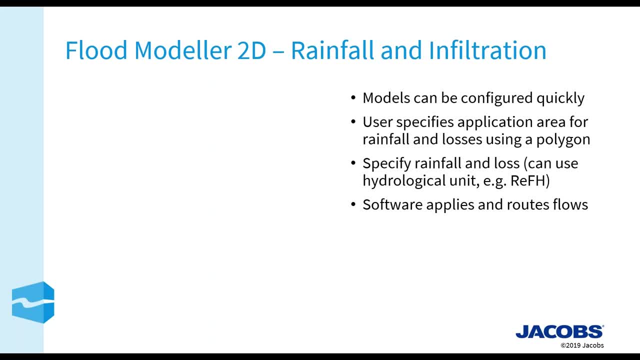 noting: you apply both a rainfall. you can apply the input to the model. you can also specify an infiltration so you can use the green out message and then you can apply the rainfall data to the hydraulic model. it's worth noting: you apply both a rainfall. you can apply the input to the model. you 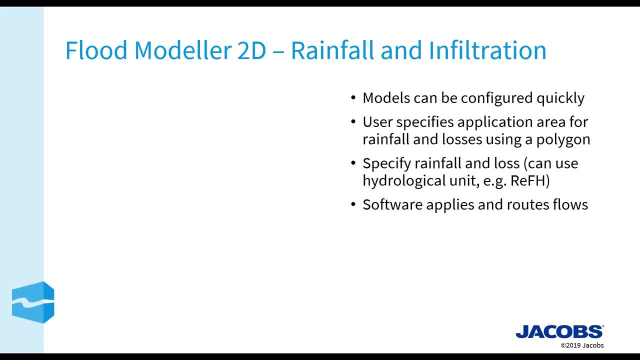 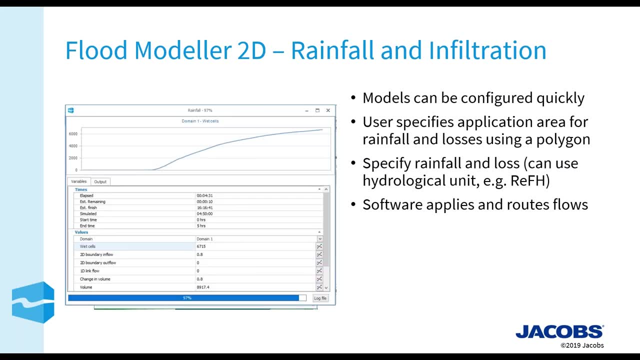 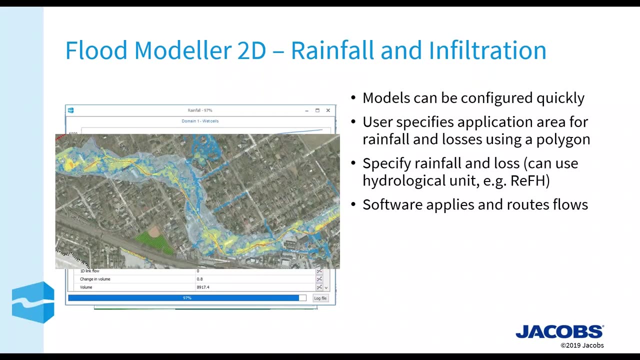 to specify an infiltration to the soil. once you've specified the location, your rainfall and infiltration will be applied over. the hydraulic model will be run, it will apply that rainfall and route that flow over land and eventually you'll end up with a flood map so you'll be able to animate how the water flows. 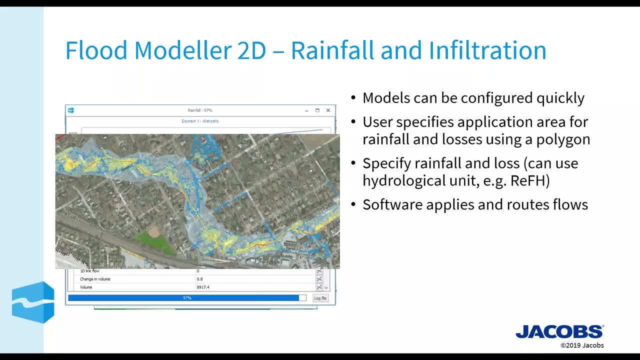 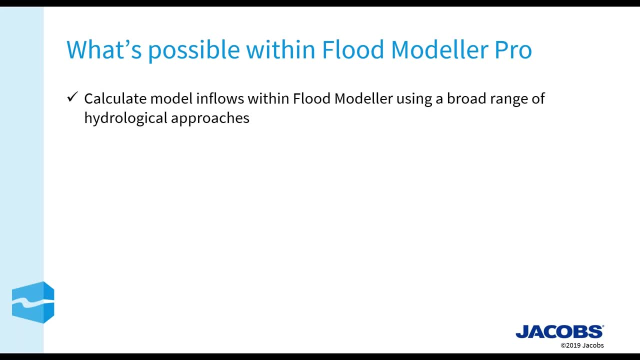 through your 2d model where it accumulates and where it's stored. so just to quickly recap what's possible with flood modeler from a hydrological perspective. the software allows you to calculate inflows to your models, calculate boundaries using a broad range of methods and it's all built into the 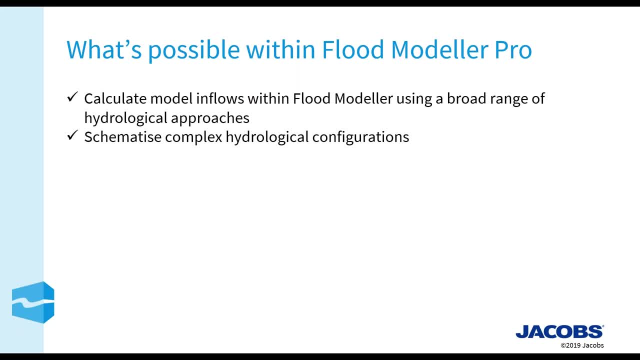 software, so it's fully integrated into what you're doing. the software is flexible enough to let you schematize complex hydrological configurations, so it doesn't matter how complex your river network is or what your study demands are. flood model allows you to cope with them. you can swap your boundaries. 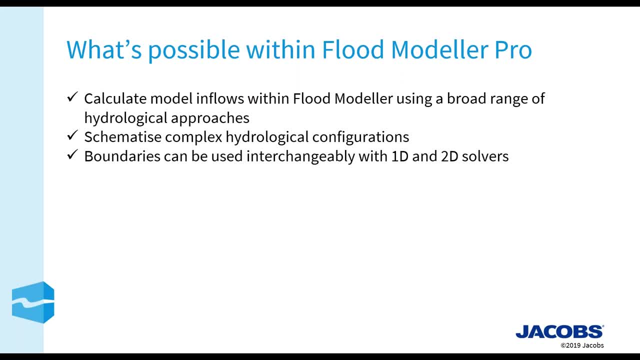 from 1d to 2d solvers easily. so if you decide you your 1d model isn't giving the results you need, it's not providing the outputs you require, you can readily swap to a 2d solver or a combination of both. we've set up workflows in the 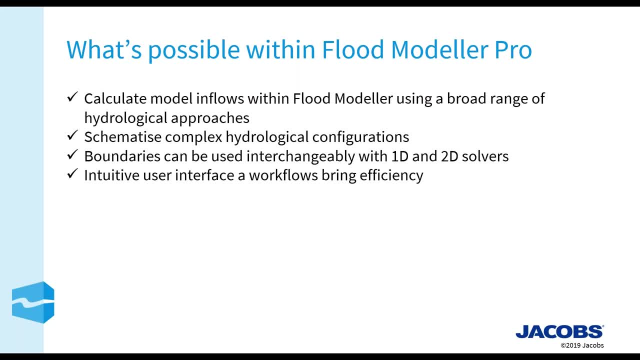 software to make this easier for you. so when you're doing RFH modeling, the workflows are there to step you through: importing the catchment descriptors, specifying the rainfall and then connecting that into your 2d model, running your model and then post processing the results all in one. 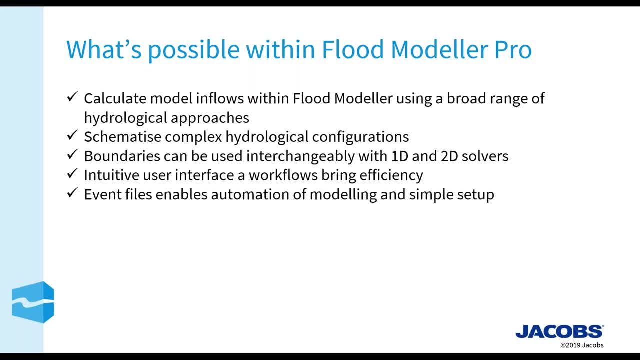 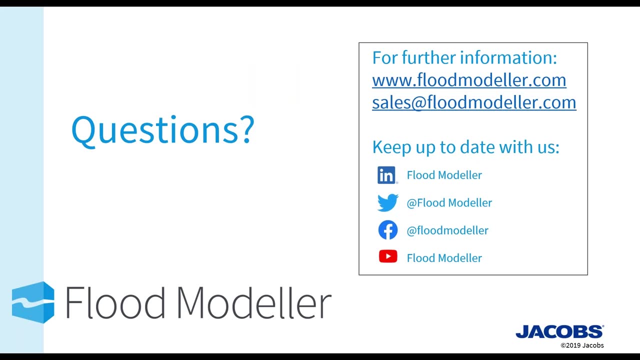 platform and the event file tool allows you to bring simplicity to your modeling. it makes it easier to set up multiple runs, lots of simulations and make the most of the automation tools built into flood modeler. hope that's given you a broad overview of how you can use flood modeler in in hydrology. you.